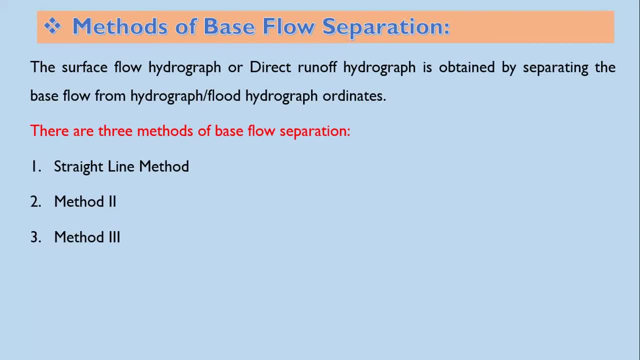 Months together also, and that flow is called as base flow. So the total hydrograph is called as hydrograph, flood hydrograph or storm hydrograph. And if this base flow is separated from the hydrograph, in that case the hydrograph is called as surface flow hydrograph. 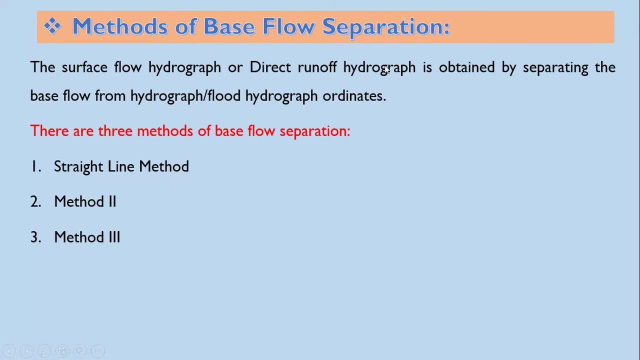 Also called as direct runoff hydrograph, known as DRH direct runoff hydrograph. so for getting this direct runoff hydrograph, base flow is separated from the hydrograph Right. So there are three methods of base flow separation for getting this DRH direct runoff hydrograph. 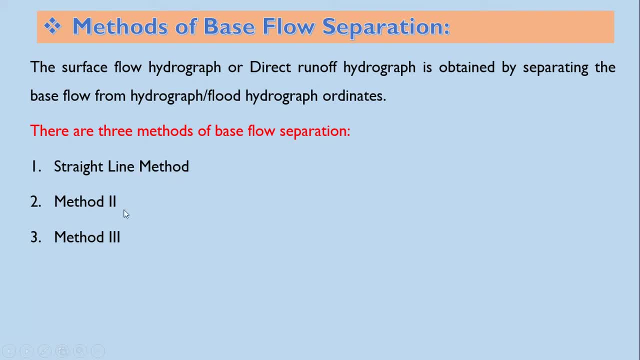 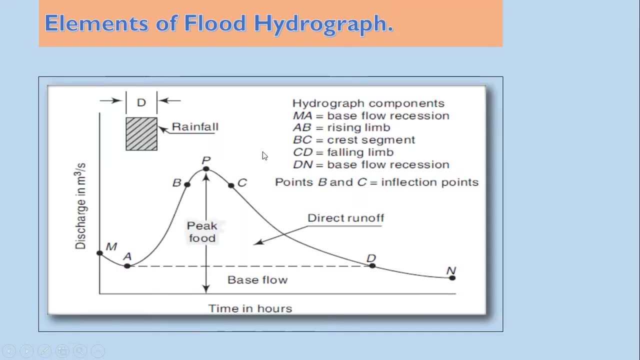 First method is called as straight line method. second is called as method number two. No name is their facial name. third is called method number three. We shall discuss one by one. So these are the elements of hydrograph, what we have discussed. So this hydrograph is called as a hydrograph. 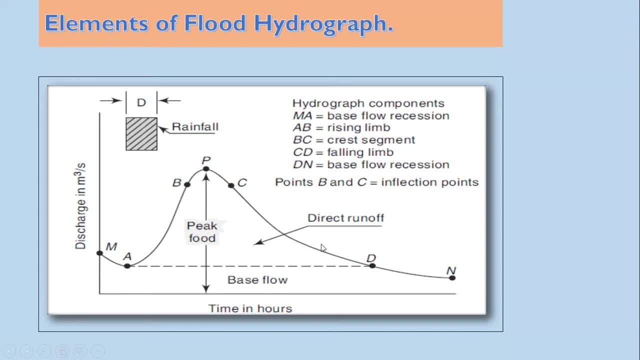 Flood hydrograph or storm hydrograph. this total is called as hydrograph. This get it understood. This is very important concept. This total is called as hydrograph or flood hydrograph or storm hydrograph, And this bottom part is called as base flow- natural flow. if this base flow is separated, 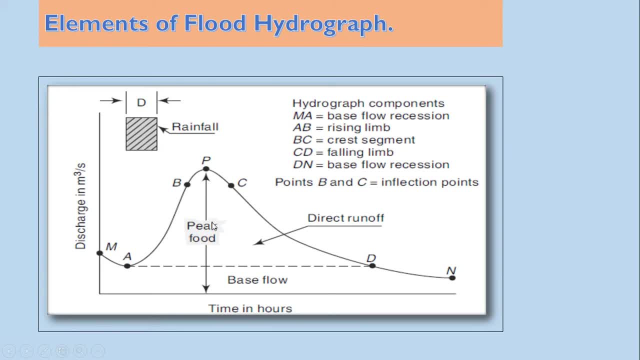 whatever hydrograph Remains, it is called as a DRH, direct runoff hydrograph and runoff under this Is called a direct runoff hydrograph. if you find out the volume of this area, of this area under this, will you direct runoff hydrograph. Now method number one. it is called as straight line method. 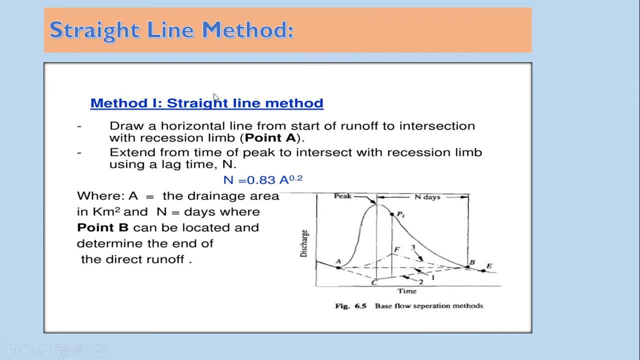 It is called as straight line method. So in this method, Separation of base flow is achieved by joining with a straight line The beginning of the surface runoff to a point on the recession limb representing the end of direct runoff. So in this straight line method, what is done? 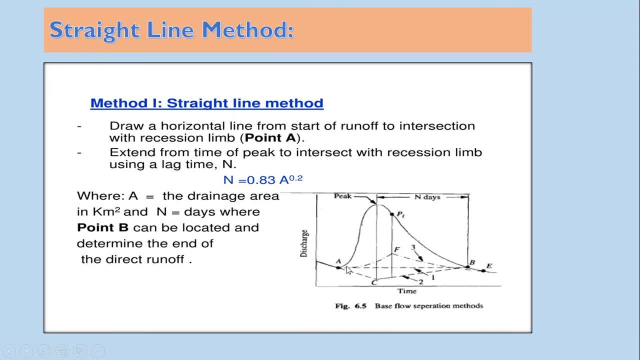 The beginning of the runoff, that is point A, join with End of surface runoff with the straight line and that's why the method is called as straight line method. So in case of this straight line method, It is easy to know the point A from where There will be built up of the runoff. 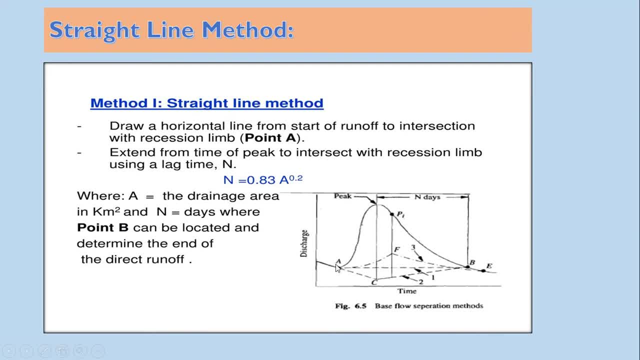 So this point A, very easily one can find out. that is starting point. But the question arises, the difficulty arises, how to locate this point B? it may be here, It may be here, It may be, it may be anywhere in this portion. So how to locate this point B? 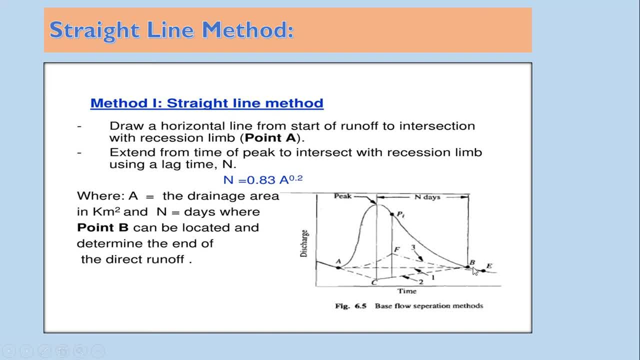 So hydrologist has given relationship In terms of: in this n equals to 0.83, a to the power: 0 point. So from this ordinate, that is the ordinate at peak Dicha, it is plotted and from this endage is measured. From this endage is measured and that will represent, that will show. 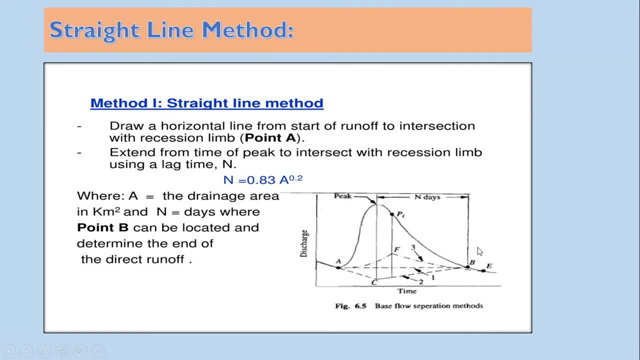 the position of point B. Hope it is clear. So n is n equals to 0.83, a to the power: 0.2, where n is number of days. A is the area of catchment or base in in terms of square kilometer. So now, with this relationship, the point B can be located and determine the end of the direct runoff or surface runoff. 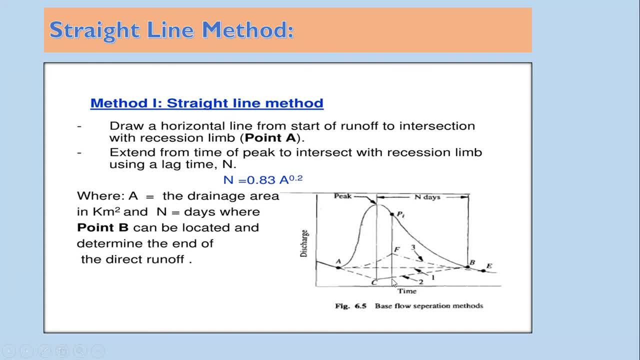 Joining point A with point B, one can get the straight line And the portion below this. this complete portion, the portion below this will give you base flow. So here you will get various ordinate, different ordinate of this base flow and if these ordinate are deducted from the ordinate, the total ordinate of 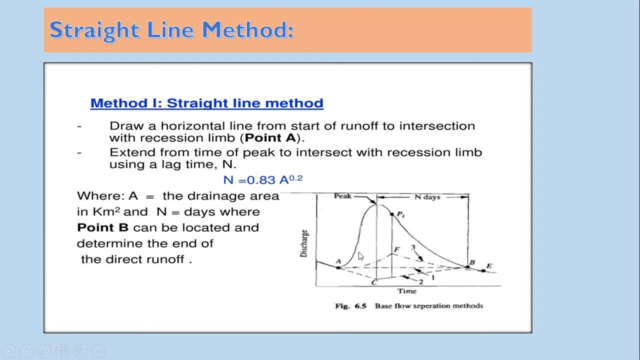 Hydrograph one will get ordinate of surface runoff, or you can say D or H. The portion about this dotted line is called as DRH, direct runoff. so this is method number one. hope it is understood. very simple. so what is done in case of this? very 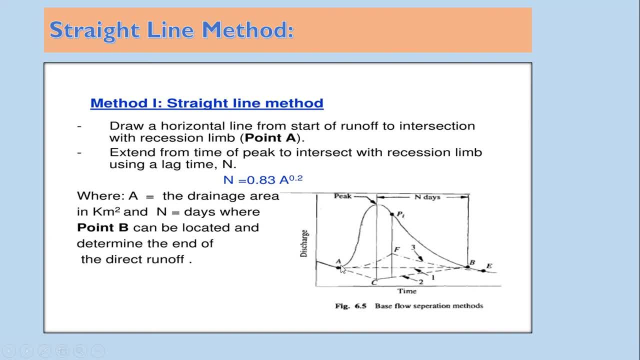 first point a is located. right, it is nothing but starting of the run-up. then point b is located. these two points are joined with the straight line. the portion below this will give you base flow. now here there is a difficulty to locate exactly locate this point b, so it 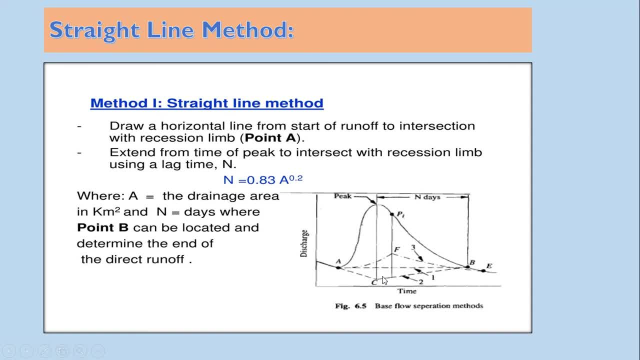 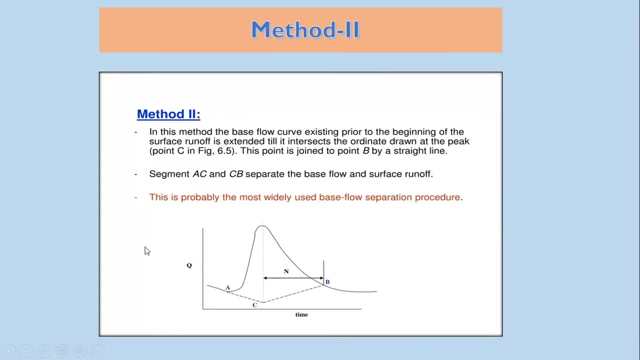 is located n days from the ordinates at the peak. how this end is calculated with this relationship: n equals to zero point eight, three a to the power, zero point two, and then it is measured from here. so this is regarding method number one. so method number two in. 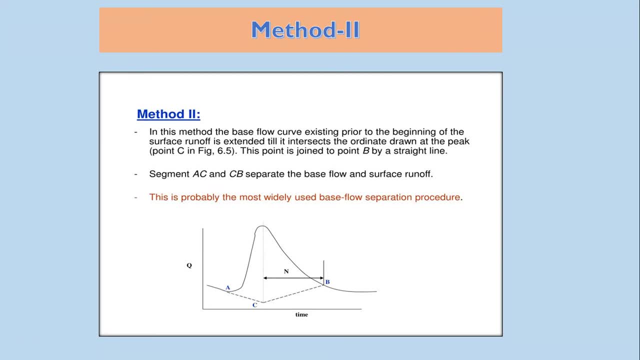 this method. second method: the base flow curve existing prior to the commencement of the surface and north is extended till it intercepts the ordinate drawn at the peak. this point is joined to point b by a straight line, segment ac and cb. segment ac and cb demarcate the base flow. 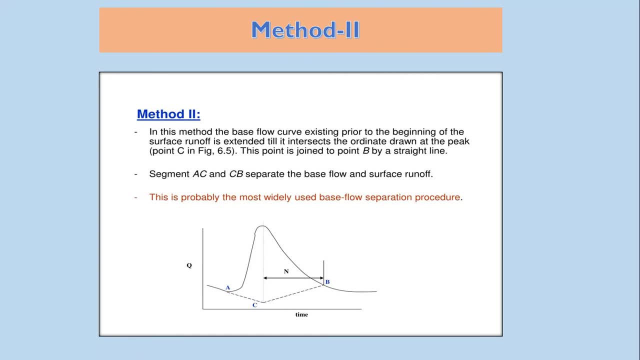 and surface, and this is probably the most widely used base flow separation method. this is probably so what is done in case of second method? now here no question of b. very easily you can locate. so in case of this method, first you have to show the ordinate and the peak, so this is the order at the peak then. then what is done in case of this? 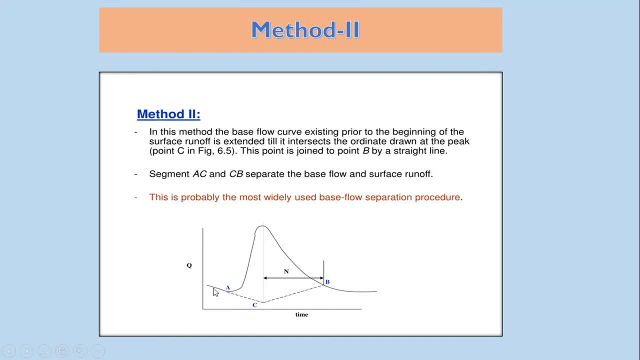 the base flow curve existing prior to this point. beginning of the surpresa. now point a. it is extended till it joined to the order rate at the peak. let this point as a point c. then a is joined with c with straight line, c is joined with point b with straight line. the area below this segment, ac. 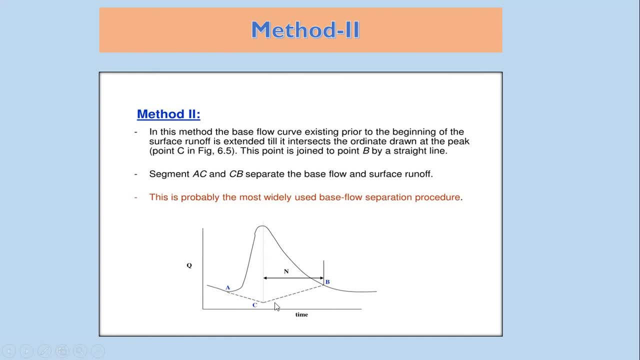 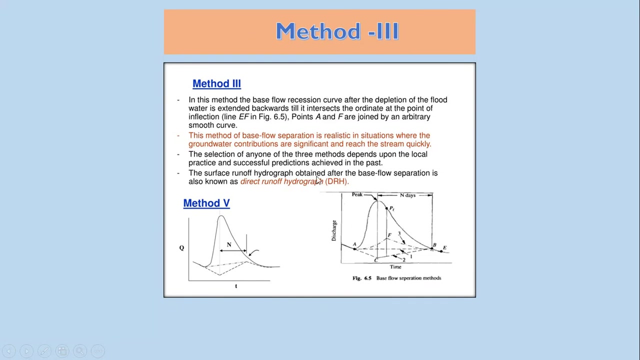 and CB, so this area will represent base. this is the most widely used method. this method is as treated as a more accurate with compared to the first method, as well as third method also. so this is regarding method 2. hope you understood it. now, coming to method number 3, no patient name is given in case of this. 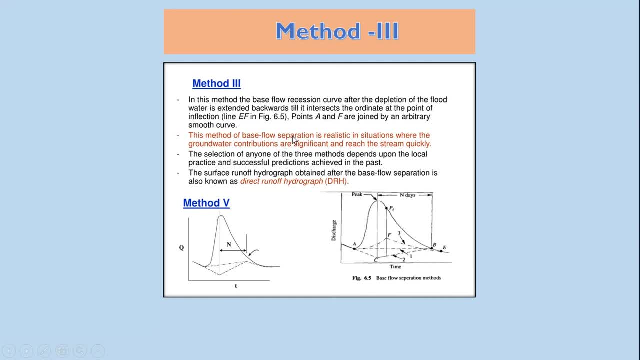 method number. what is encased of this method number 3? so in case of this method number 3, the base flow recession curve after the depletion of flood water is extended backward, the base flow curve, part of recession curve after the depletion of the flood water is extend. 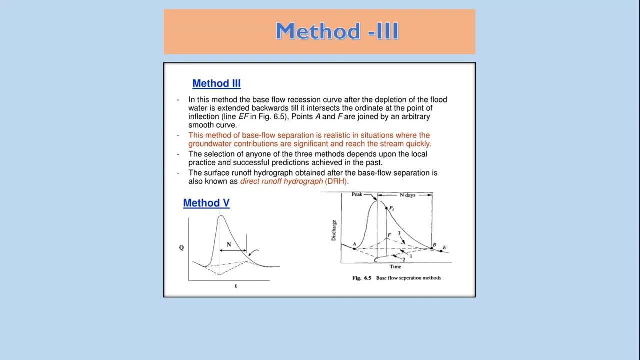 backward till it intersect the ordinate at the point of inflection. now, here the ordinate at the point of inflection is considered. in the previous two methods we have considered ordinate at the peak, but here we have to consider ordinate at the point of inflection. point a and f, let it as a point f. point a and f are joined.